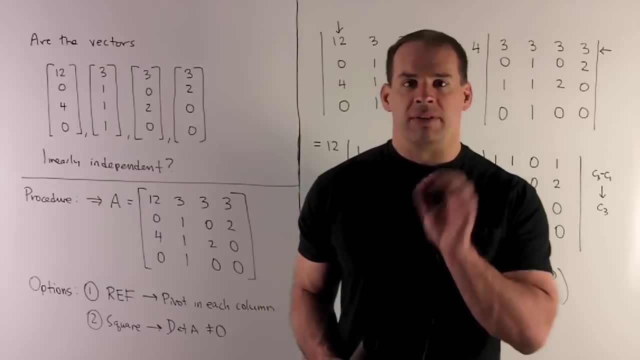 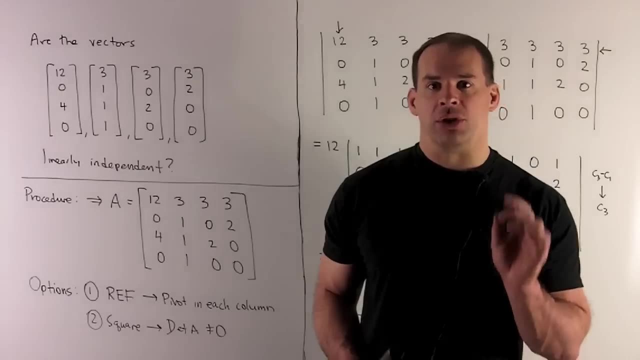 we have a square matrix, so the quick way to check whether you have a pivot in each column is just to take the determinant. If the determinant is non-zero, you have a pivot in each column and you're linearly independent. If not, then you'll be linearly dependent. 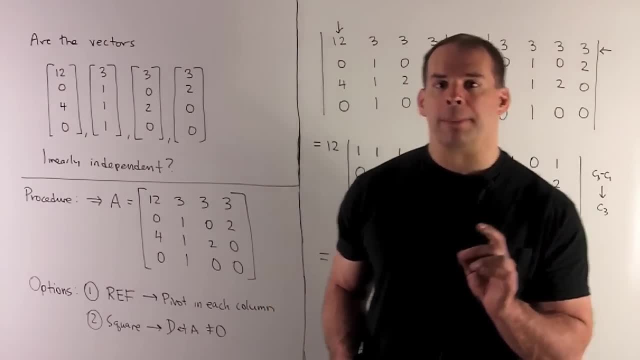 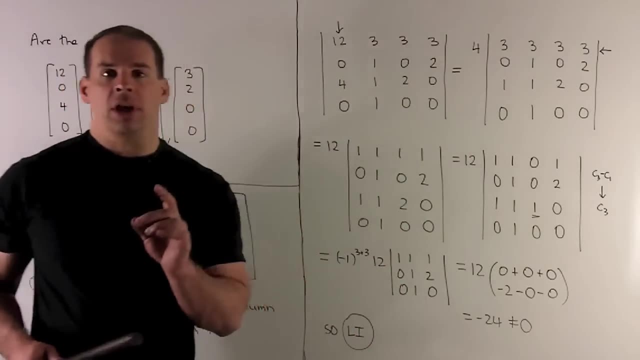 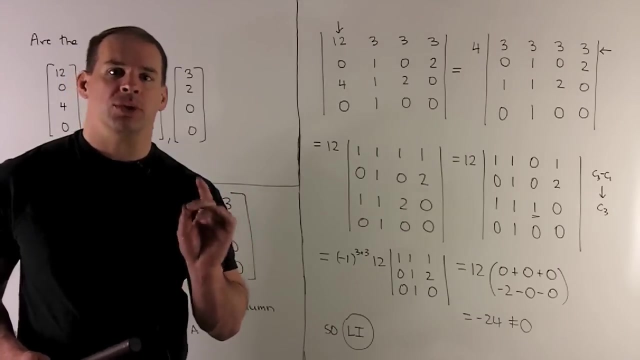 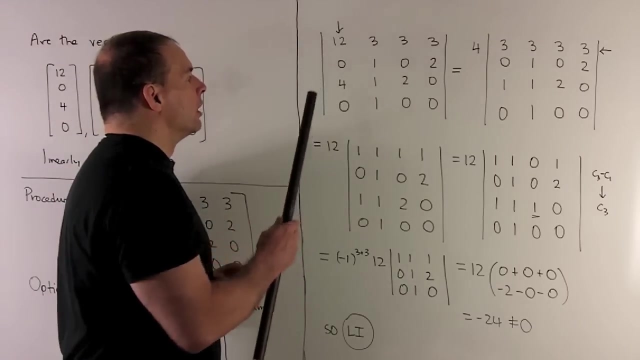 so that means determinant will be zero. We're going to put determinant in bar notation. What can we do Here? we're going to do both row and column operations, just to get used to using them both together, although here we won't do very much. First operation: I'm going to factor a four out of column one. 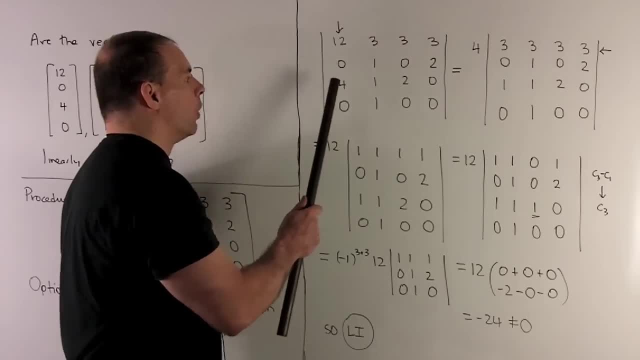 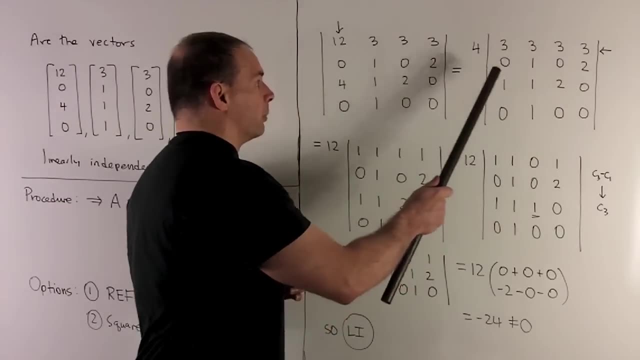 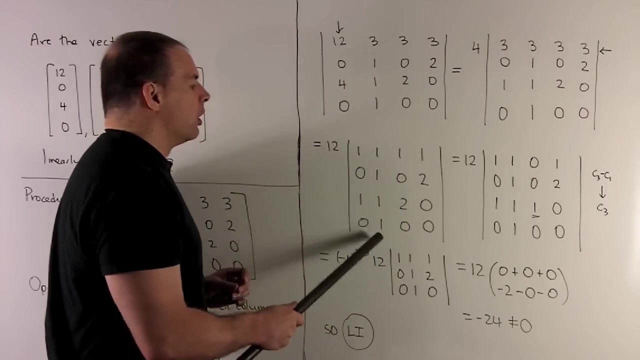 I'll bring the four in front and then this is going to turn into three zero, one zero. This operation. we can factor a three out of row one That'll put a three out in front to give us a 12, and then I get a row of ones. Now we could do a cofactor expansion off of. 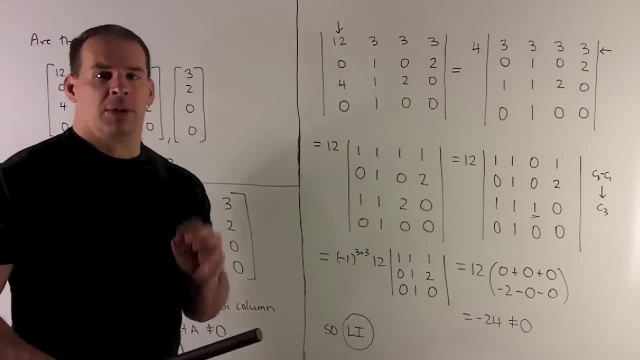 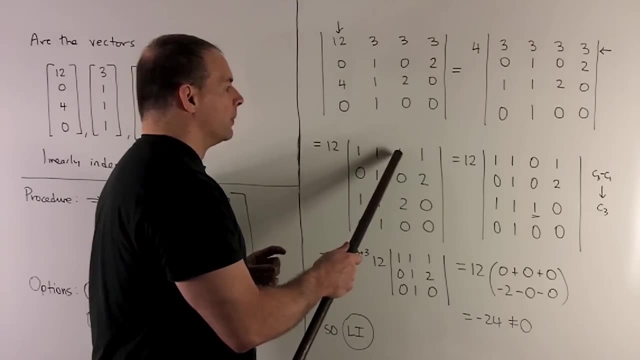 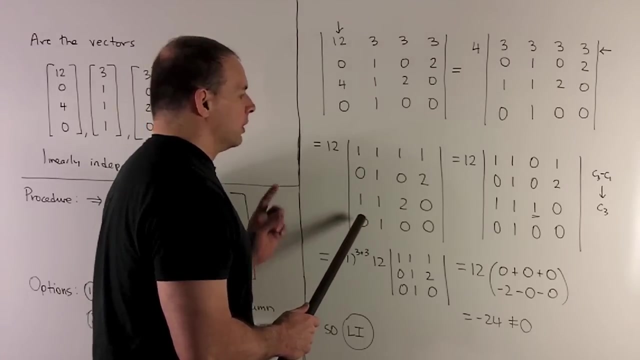 this one here, since we have all zeros. that would be good, but let's just do one more column operation. I want to turn this two into a one and this one into a zero. What I'll do is we'll take column three, subtract off column one. I'm going to do that. I'll. 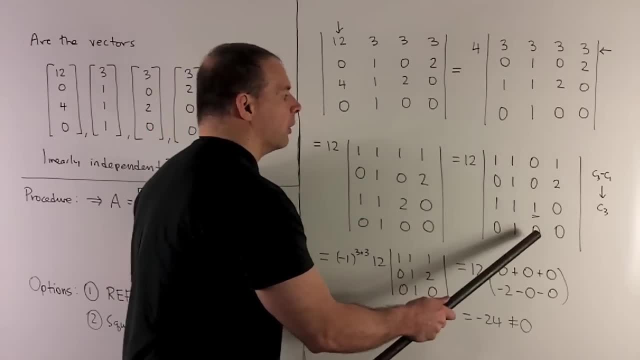 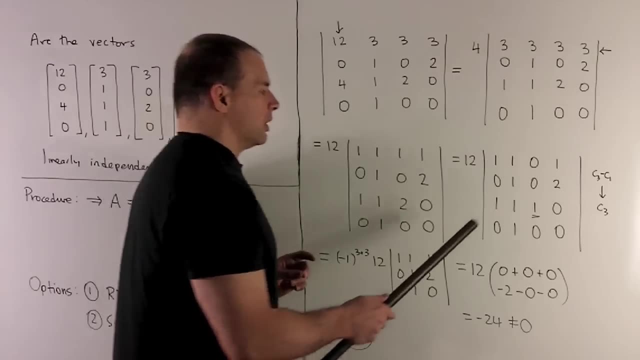 It's going to give me exactly what I said. We'll have 0, 0, 1, 0.. Now I can do a cofactor expansion off of this point here. So what's going to happen? We're going to take our row and column number, add them together. 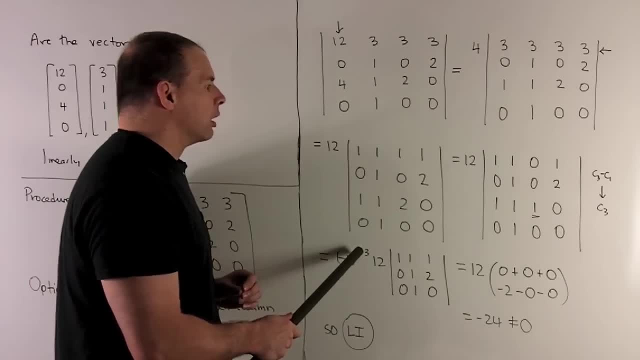 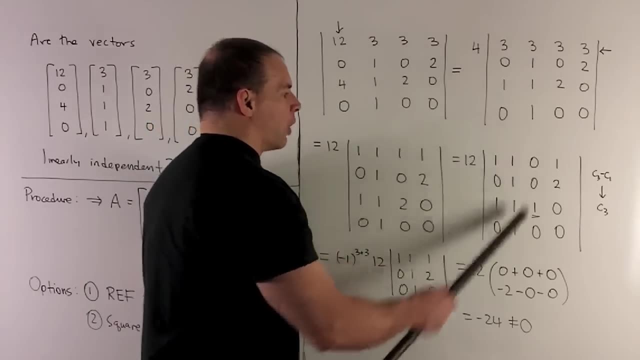 So it's 3 plus 3.. Take minus 1 to that power. The 1 here would come out, but 1's not going to do anything. We have the 12. And now I'm going to cancel out the row and column. take the determinant. 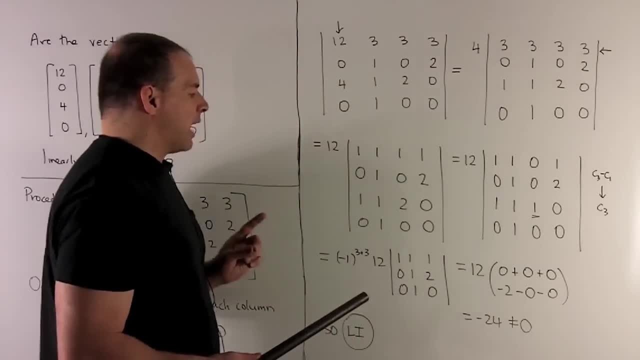 So we're going to get the minor for this entry. Now that gets me down to 1, 1, 1, 0, 1, 2, 0, 1, 0.. Then you have the options. 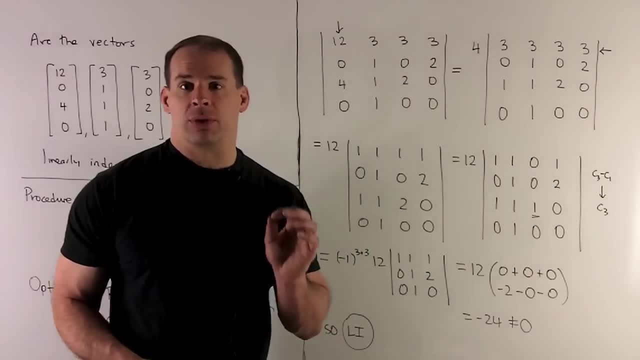 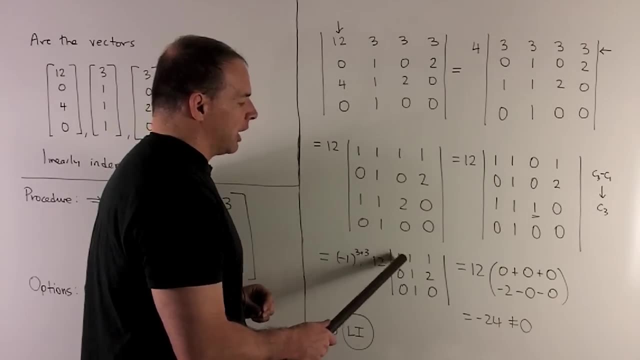 You can either go with your diagonal way of computing the determinant of a 3 by 3 matrix, or you can just note: okay, you have a 1 here, so another cofactor expansion is just going to get you. okay, you just do your 2 by 2, you're going to get a minus 2.. 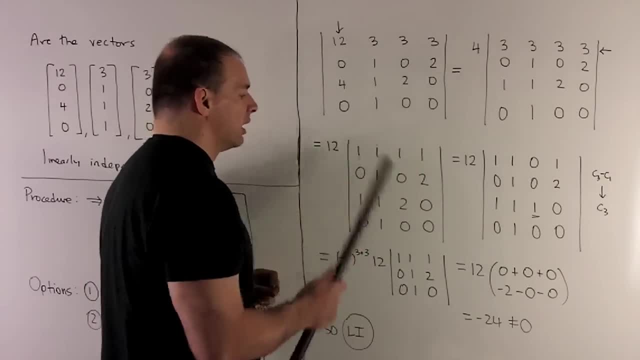 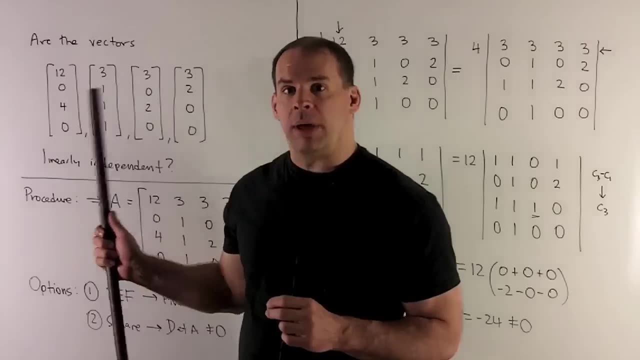 So at the end of the day the determinant of our 4 by 4 matrix is going to be minus 24.. That's not 0. So our set of that is going to be linearly independent.